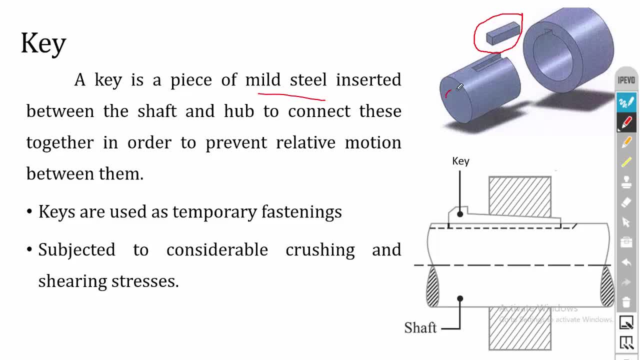 motion and because of the key, the torque transmitted from the shaft is transmitted to the pulley or gear. So the key is a critical element and the key is a temporary fastener. So if you want to remove the pulley or gear from the shaft, then you can remove the key. 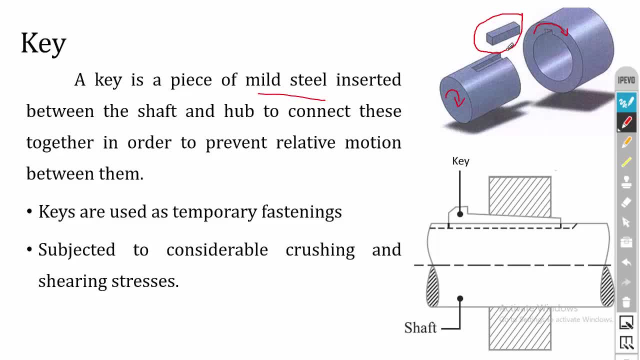 and you can remove the pulley. And second one: the key is subjected to crushing and shearing stresses. So, because of the relative motion between the shaft and the hub, the key is subjected to shear stress and because of this area, half of the you can see here. so because 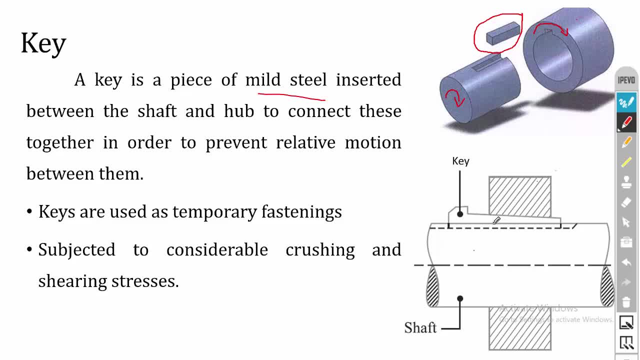 of the motion between the shaft and the hub, the key is subjected to shear stress. in this point And at this area, the key is subjected to crushing stress. So because of the torsionary motion of the shaft. So, while designing the key, these two factors should be considered. 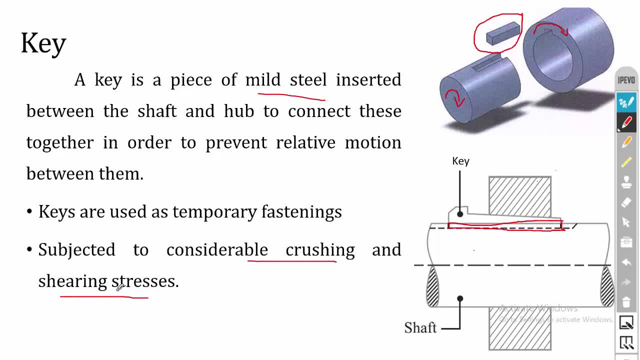 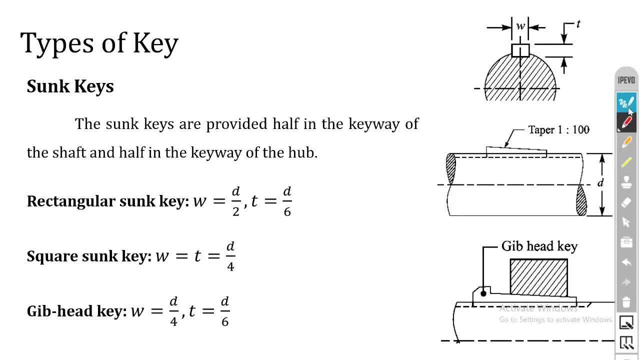 The first one is crushing stress and the second one is shear stress. These two should be considered for selecting the dimensions of the key. So there are many types of keys are there. The first and most common one is a sunk key. So in the sunk key you can see this image- the half of the part of the key is inserted. 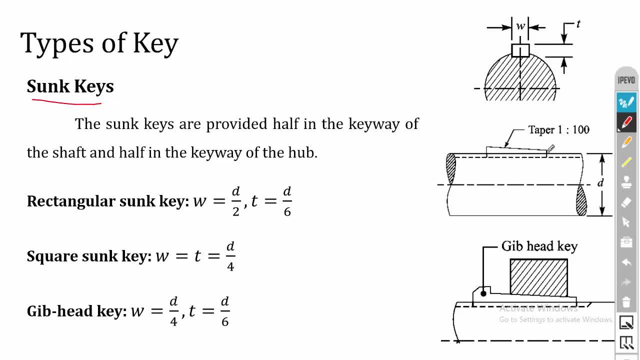 in the shaft and the remaining half is inserted on the hub. And for rectangular sunk key the width is half of the diameter and the thickness is 1 by 6 into the diameter. So here D is the diameter of the shaft. In the case of square sunk key, the width and thickness is same. 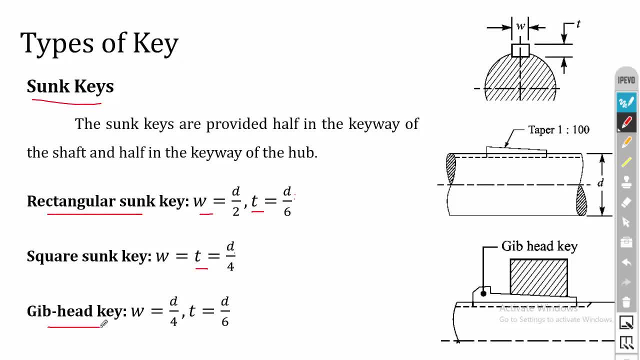 And that is equal to D by 4.. Then for zibhead key, it is almost like a rectangular key. The only thing is that the head is in the front part of the key. So this head is used for easy dismantle of the keys. 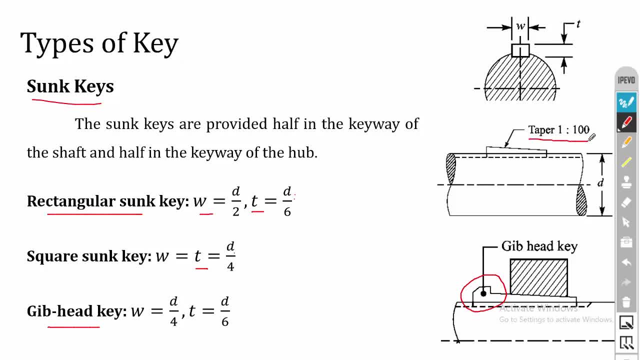 So in this sunk key the number of tapas are 1 by 100. So you can see a small number of tappa in key length. So tappa is 1 by 100. So the sunk key, half of the key is on the shaft and the half of the key is on the hub. then the next key. 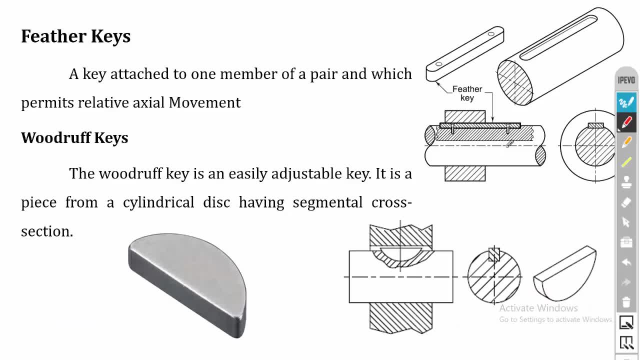 is a feather key. so in the feather key the key is attached on the shaft and it is inserted on the hub. ok, so you can see the holes. so the key is screwed on the shaft, you can see that, and the hub is free to move in the axial direction. so this feather key allows the free. 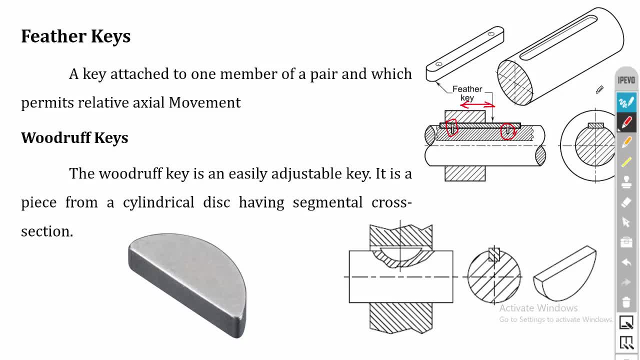 movement of the hub in the axial direction, but in torsionary direction. it will not allow relative motion, so it will transit the torque. The next one is Woodruff key. so it's a cylindrical disc, half of the cylindrical disc. you can see that the disc is inserted on the shaft and some of the projections are inserted on. 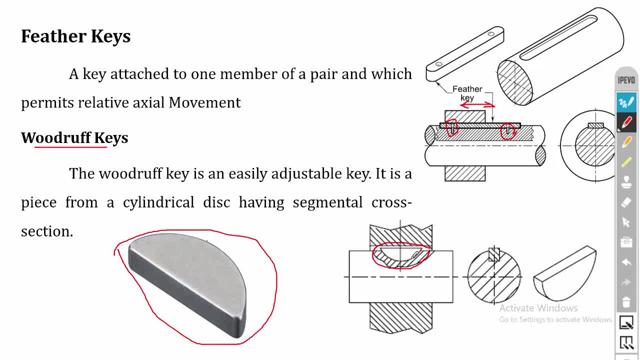 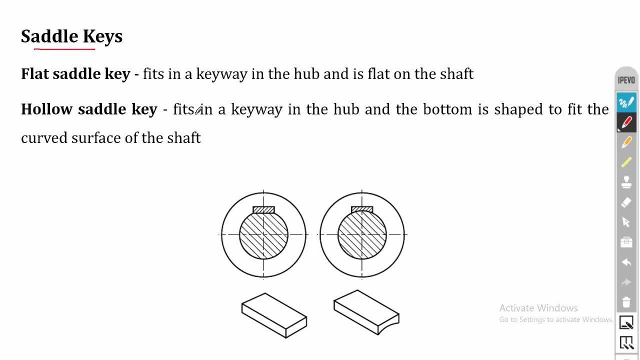 the hub so this key automatically adjust to avoid some misalignment or irregularities in hub. So that is why woodruff key is used and the next one is saddle key. so there are two types of saddle keys are there. one is a flat saddle key and another one is a hollow saddle key. 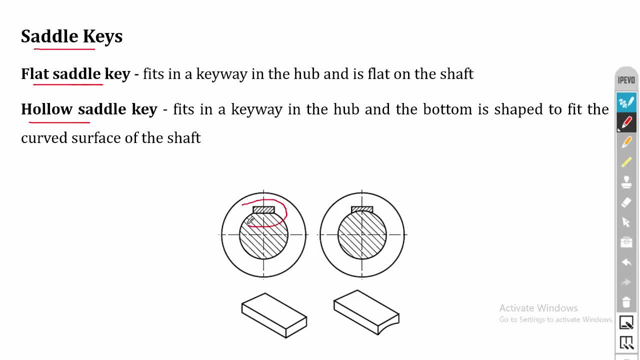 so in the case of flat saddle key it is a rectangular cross section and there is no curve linear section on its surface. so the top of the section is connected with the hub and the bottom of the flat surface is connected. It is allowed to rub on the shaft and in the case of hollow saddle key, the top surface. 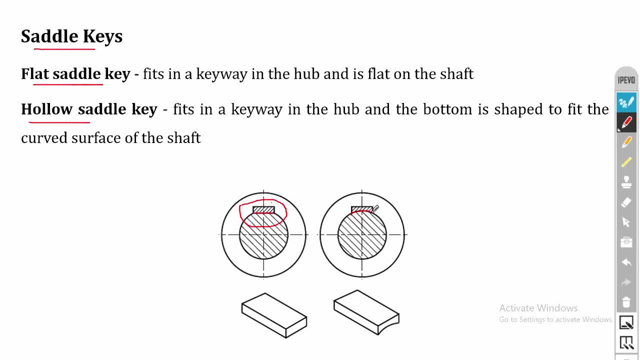 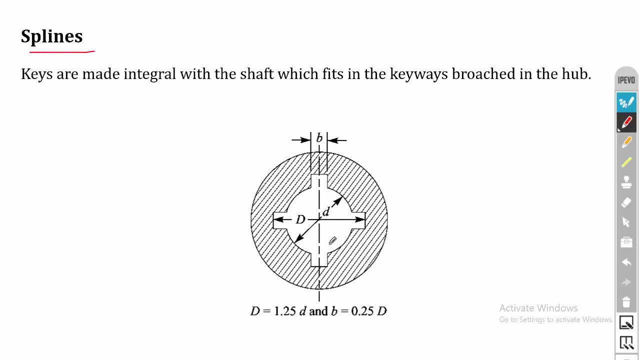 is a flat and the bottom surface is a curved surface, and this curved surface is fixed on the shaft and the flat surface is inserted on the hub, Then splines. so in the case of splines, the keys are made integral with your shaft and the keyways are broached on the hub. you can see that this is a hub and the centre part. 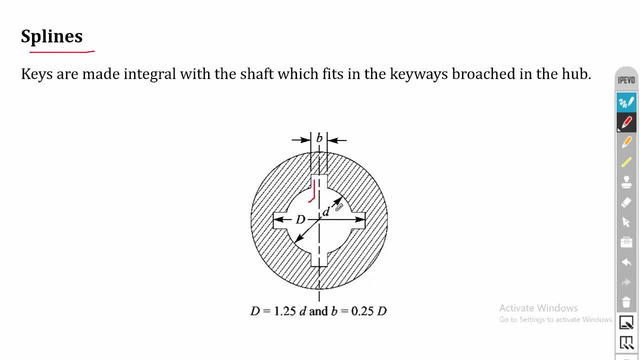 is a shaft, so this key is made integral with the shaft, so this kind of shafts are called as splined shaft. so here the diameter of the spline is 1.25 times the diameter and the thickness of the spline- that is, width of the spline- is 0.2 times the diameter. now coming 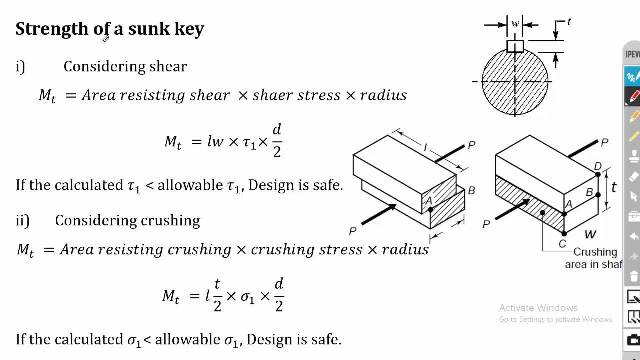 to this design of key. so, as i told earlier, the keys are subjected to two stresses: one is shear and crossing stresses. so in this subject we are going to design only the sunk keys. ok, so first one, considering shear. you can see that. so the width of the key is w, the thickness is t. so 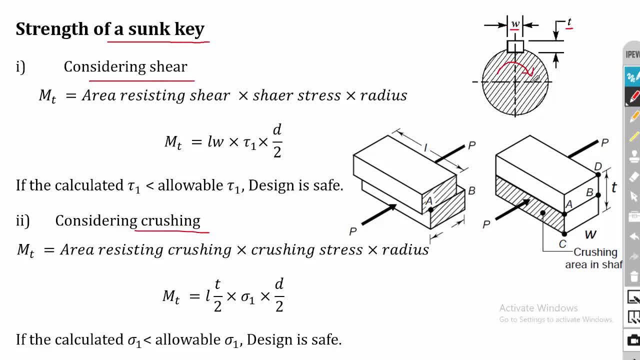 when relative motions occurs, the shaft will rotate in this direction and the hub will resist the motion in the opposite direction, so a relative motion occurs. so, because of the relative motion between two mating parts, what will happen is the half of the part is subjected to a tensile force on the right and the upper half is subjected to a tensile. 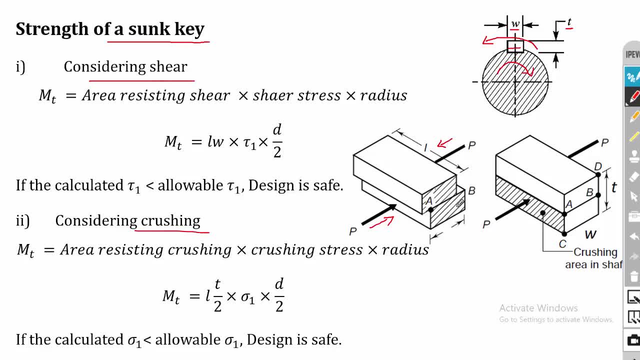 force to the left. you can see that. ok, so this is called as shear stress. ok, so the calculation is: the torque transmitted is equal to area resisting shear into shear radius, into radius of the key. So here the torque transmitted is empty and area resisting shear is w the width into overall. 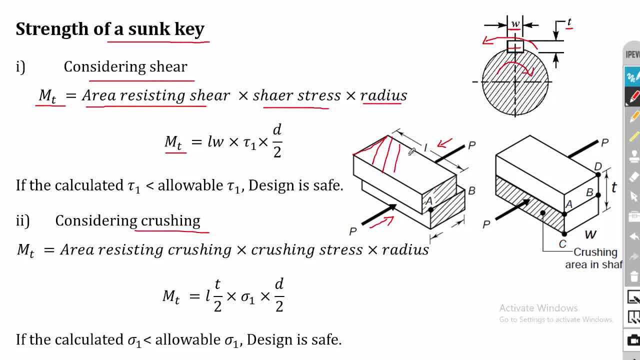 length because this area is resisting the shear, so it is l into w and the shear stress i have considered as tau one. ok, so you just consider it as tau. and the radius of the shaft is d by two. then if the calculated tau value is less than the allowable tau value, then 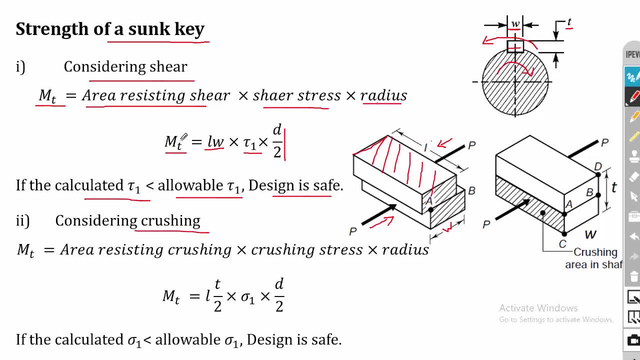 the design is safe. so i will tell you how. so, while designing a key, we must substitute the value of mt and we have to select the l and w value from the standard data, and we know the value of diameter. ok, so, after substituting everything, we have to calculate the value. 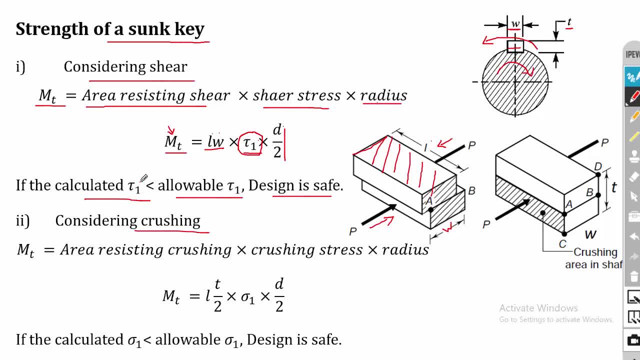 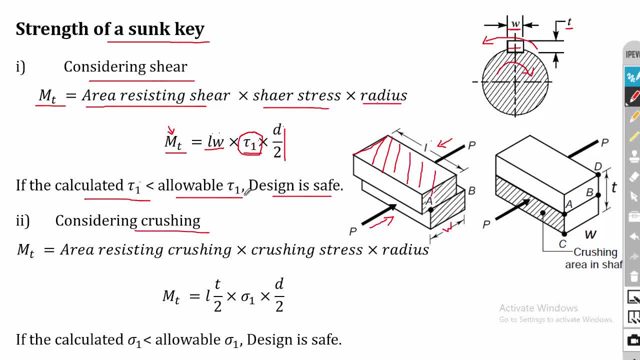 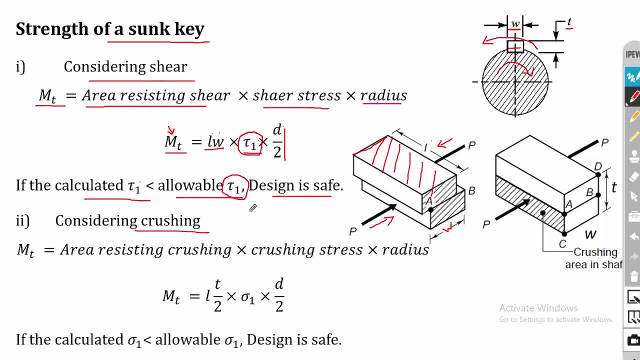 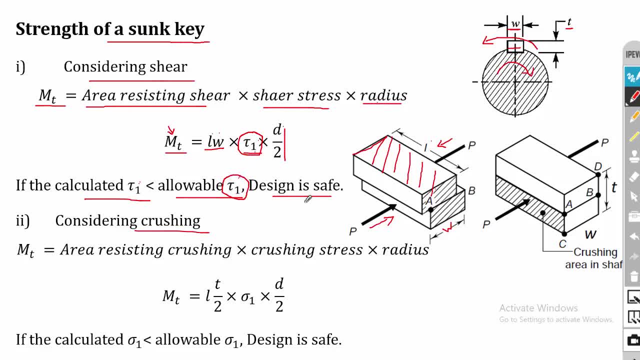 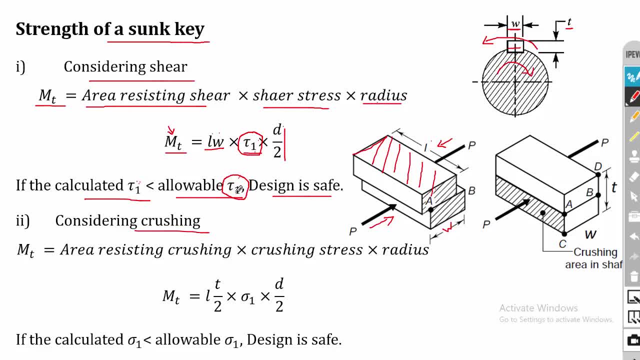 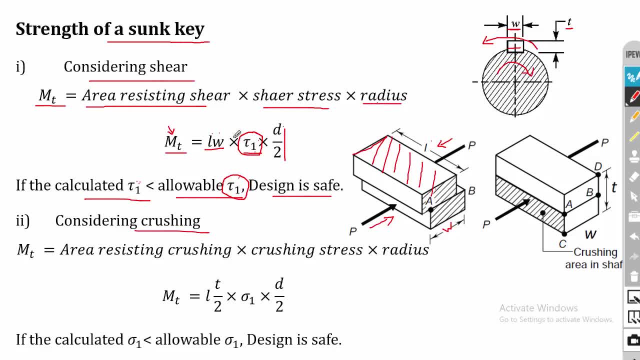 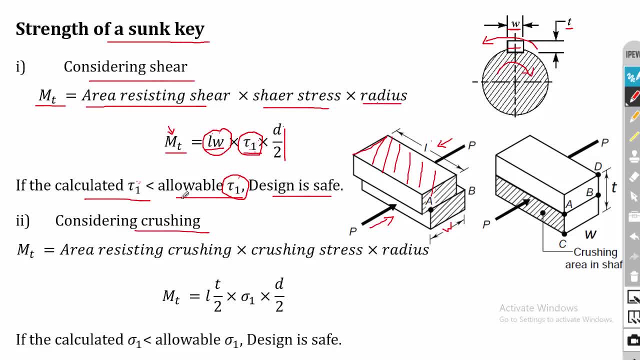 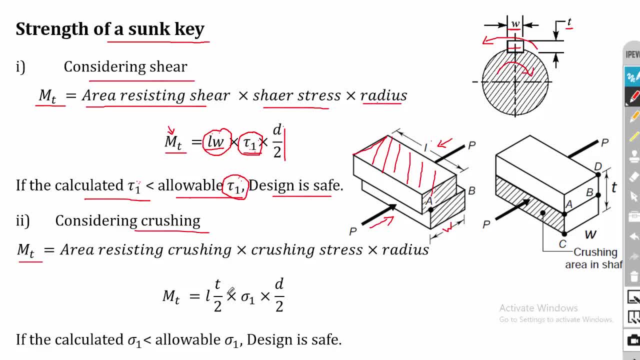 So tau one is the calculated shear stress. Then, in the case of crushing, the torque is equal to. so here area resisting shear and here it is area resisting crushing into crushing stress, into radius. So in the case of crushing, the half of the key surface is subjected to crushing. 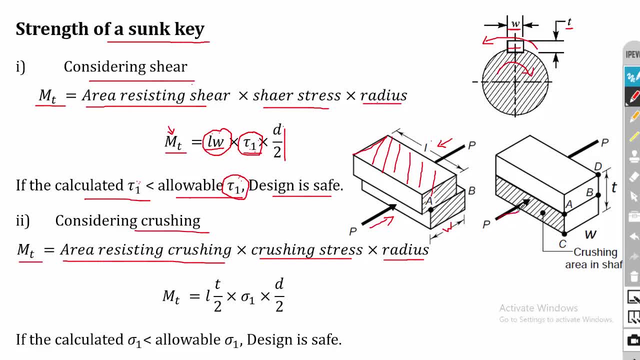 You can see that this lower part is subjected to a crushing stress because of the rotation of the shaft And the upper part is subjected to another crushing because of the rotation of the hub. So we will consider any one of the half. So I am going to consider this side. 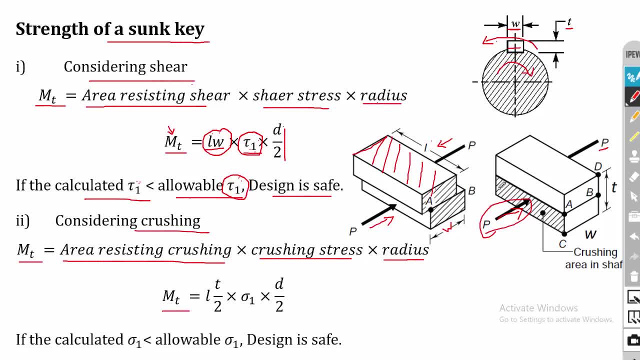 So the torque is empty and area resisting crushing is: this is the area that is resisting the crushing stress. So it is the length into thickness divided by 2, because half of the section is subjected to the crushing stress. Then the crushing stress is sigma 1 and the radius is half. 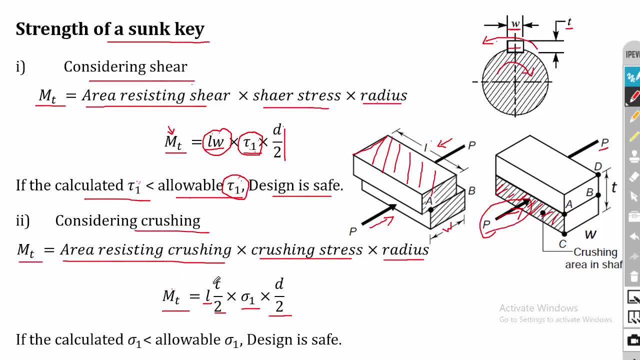 So here you have to substitute the empty value l, ie the standard length of the key. then thickness is the standard dimension and diameter of the shaft. You have to calculate the sigma 1, that is the material property of the key material. So in the case of mild steel, sigma 1 for mild steel, after considering all the factor of. 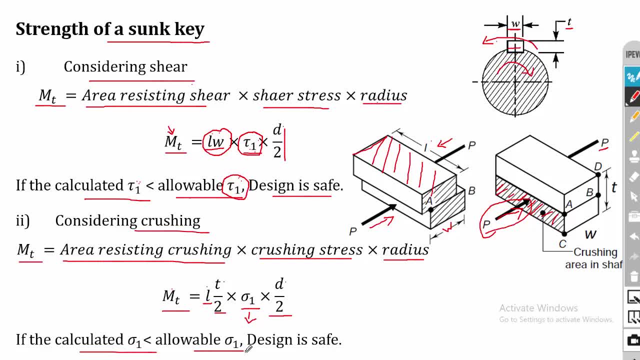 safety values is 90N per 1240.. N is very important, So the factor of safety value here is 90N per 1240. mm2.. So that is the allowable sigma 1 value for mild steel. So if your calculated sigma 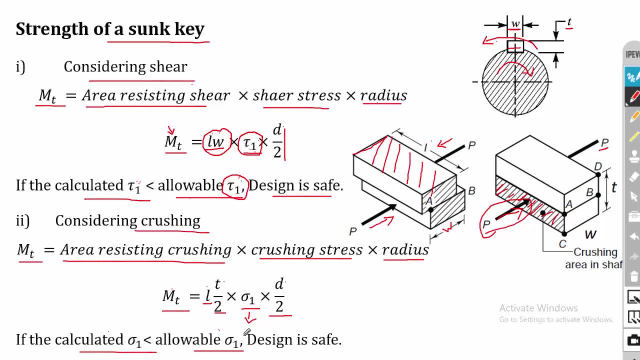 1 value is less than the allowable sigma 1 value, that is, 90 newton per mm2, then your design is safe. So if it is not less than the allowable stress value, then you have to go for revision of the key dimensions, that you have to improve the key dimensions. So 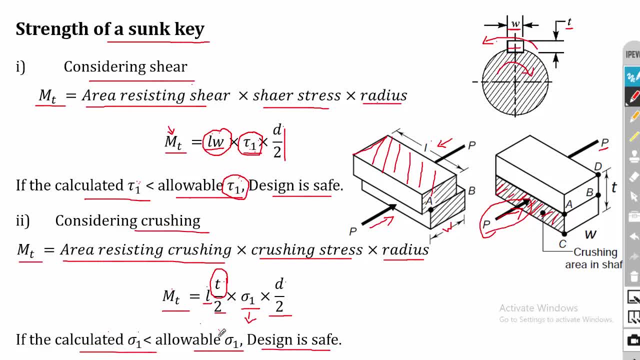 you have to increase the dimensions so that your sigma 1 value will be less than your allowable sigma 1 value. So these two factors should be considered while designing a key, and this is how you have to design the key. So now we will see how to select the standard. 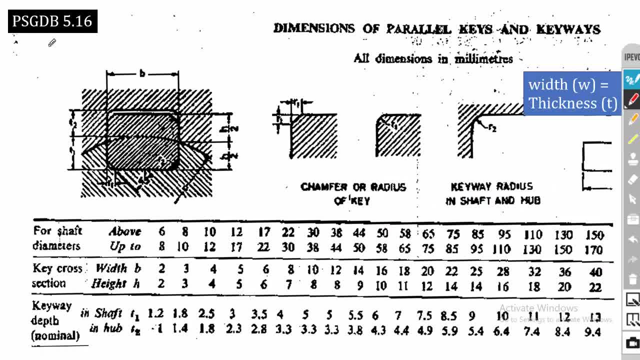 data from data book. So in the data book, page number 5.16, you can see the chart for dimensions of parallel keys. So in that the first one is for shaft diameters, and this is the key dimension, So here width is given as 0.5.. So this is the key dimension, So here width is given. 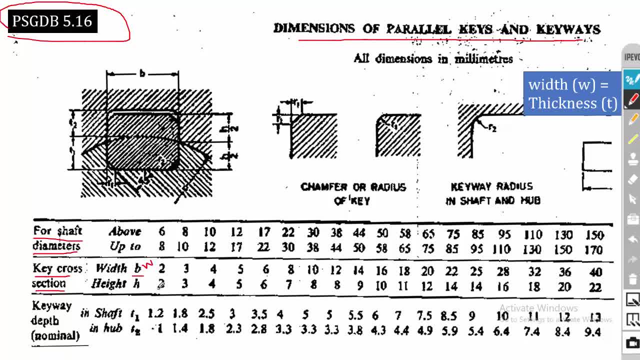 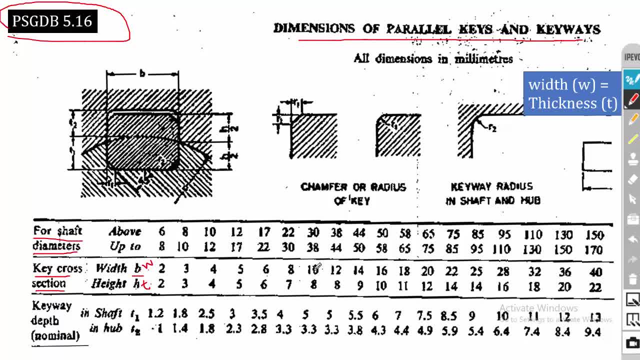 given as 0.5.. So here width is given as 0.5.. So here width is given as 0.5.. Here thisgem and width is given as0.5.. Based on the size duration, then you can check the key size value. 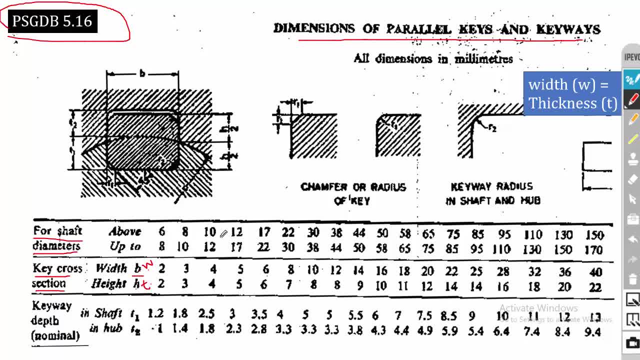 of the key dimension. For example, let us take shaft size of 6 to teeny value as well. So, and here it is 30 to 38. okay, so D, that is, 35 mm, is in between 30 to 38 mm. so for this band, your key width is 10 mm and your key thickness, that is, height, is 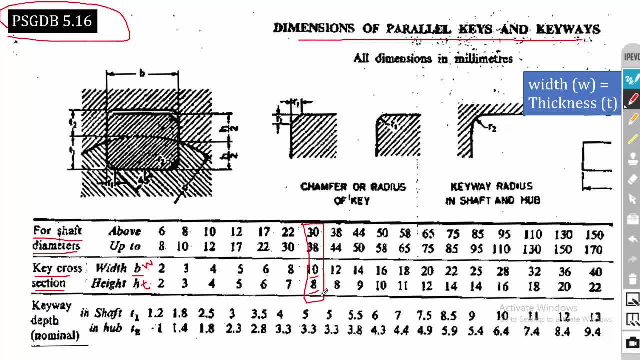 8 mm. so in the case of: if shaft size is 55 mm, then this is for the shaft size 50 to 58 mm. so your W is 10 mm and T is 10 mm. so W is 16 mm and T is 10 mm. for. 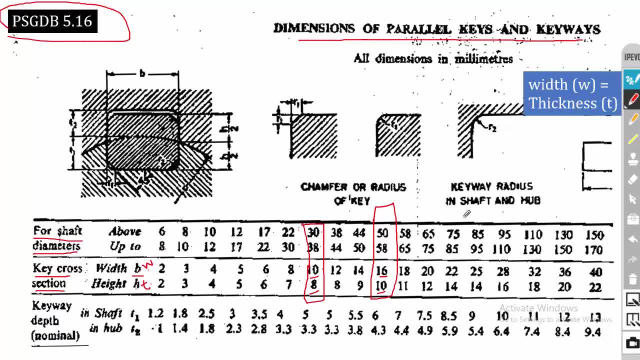 example, if your shaft size is 75 mm, you can see that there are two 75 values. are there, okay? so one is the band between 65 to 75 and the other one is 75 to 85. so my recommendation is always: you can go for higher dimension, so that the key 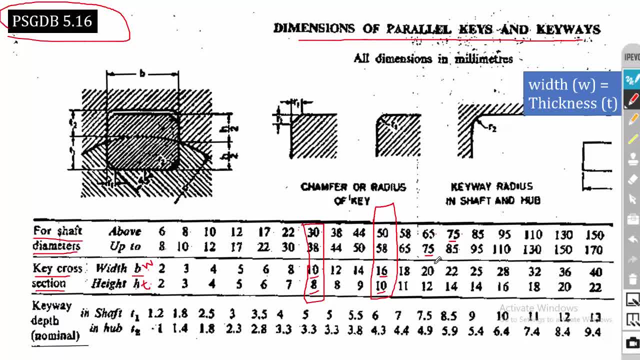 will not fail easily. okay, so go for the maximum values. okay, so go for the maximum values. so go for the maximum values. okay, so go for. So if your diameter is 75, then you can select this band. so for D is equal to 75, the key 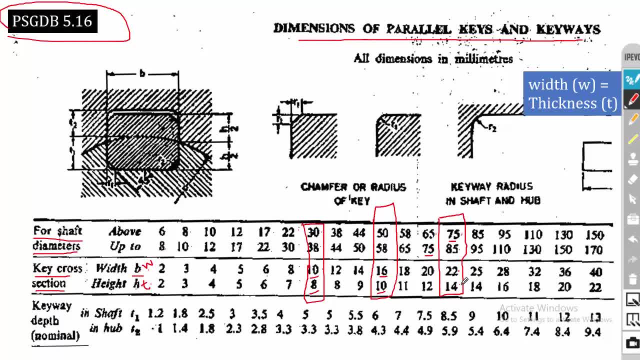 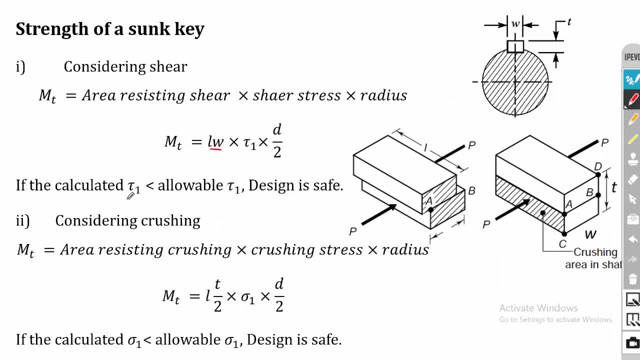 dimensions are 22 and 14, so that is, W is 22 mm and T is equal to 14 mm. So this is how you have to select the standard dimensions of key from the data book and, after selecting the dimension, you can substitute the value. in this equation, you can calculate: 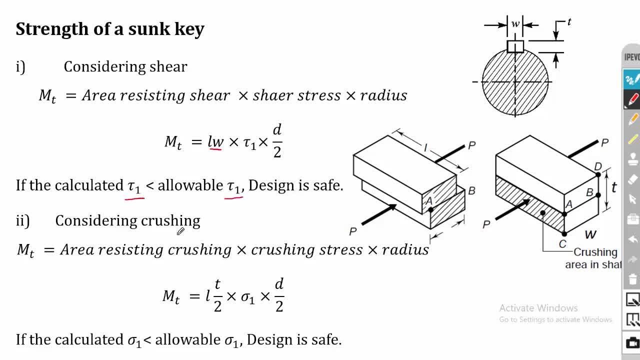 the tau value and you can compare it with the allowable stress value. in the case of crushing, you can substitute the length and thickness of the key values. you can calculate sigma 1 and you can compare it with the allowable value. but remember that if your calculated value is less than the allowable value, then your design is safe. if it is not less than, 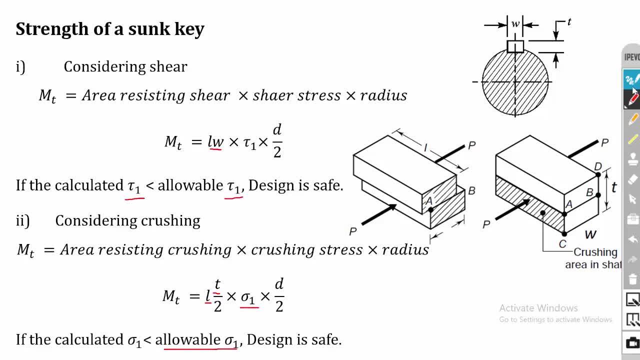 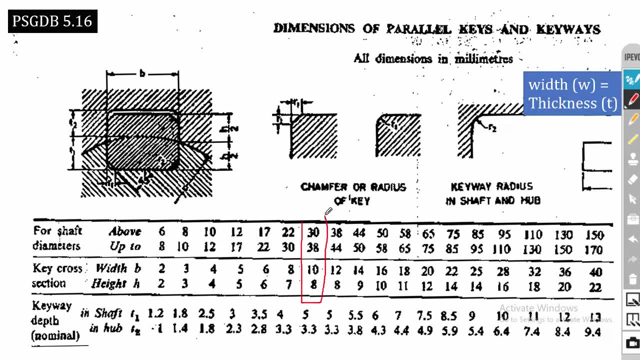 the allowable value. then you have to go for revision of key dimensions. for example, for a shaft diameter of 35, as I told you earlier, I have selected the key sizes 10 and 8, but the calculated tau value is higher than the allowable value. So what I have to do is I have to go for higher dimensions so you can select a key. 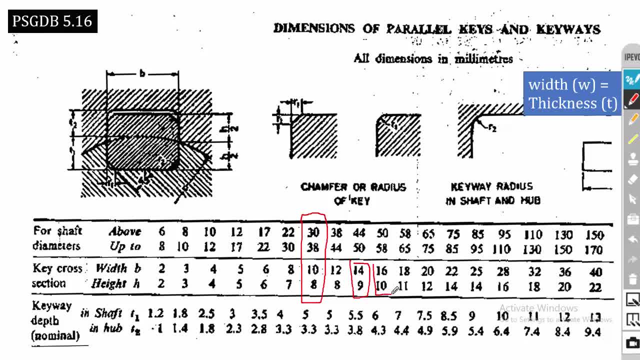 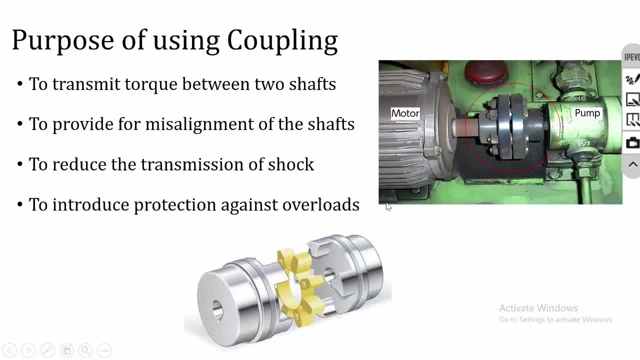 size of 14 and 9 or otherwise you can select a key size of 16 and 20, so you can select based on your stress values. so that is how you have to revise the key dimensions. Next is coupling. so coupling is used to connect two parts together. so in general, the pumps. 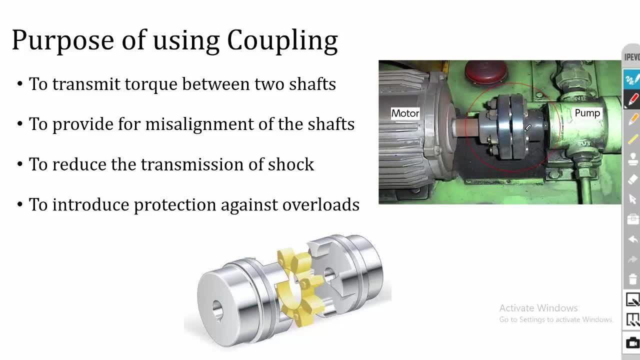 and the rotors are connected with the motor with the help of coupling. so there are four purpose are there for using coupling? the first one is to transmit torque between two shafts. so remember, consider a motor and a pump. so here the motor is generating the torque and 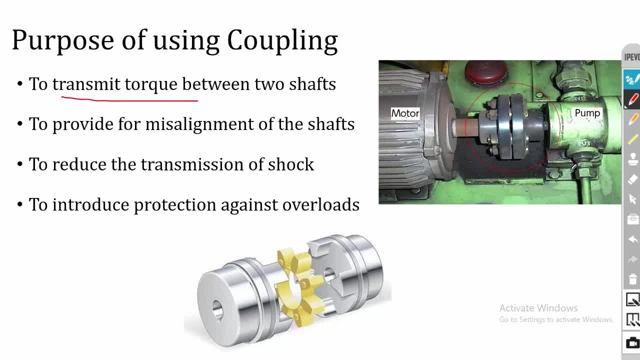 the torque generated in the motor should be transmitted to the pump. so in that the shaft of the motor is connected with the shaft of the pump by using a coupling. ok, so I think you have seen the couplings in your fluid mechanics laboratory. ok, so that is coupling. 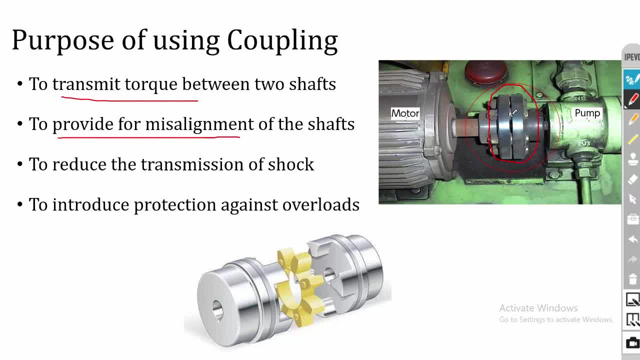 and the second one is to provide for misalignment of the shaft. so in some cases there may be shaft misalignments will be there. so that is, the shaft of the motor will not be collinear with the shaft of the pump. so in that case you can use some flexible couplings or old 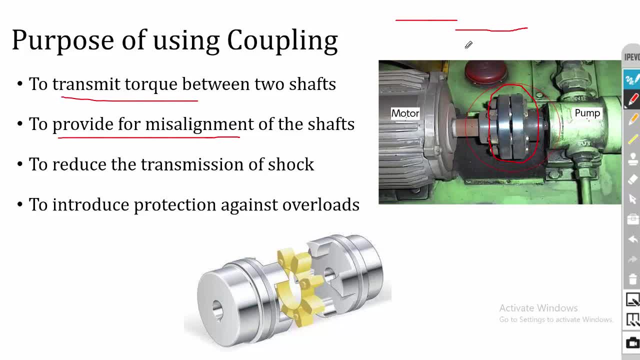 hams couplings to avoid the effect of misalignment. Then the next one is to reduce the transmission of shock. so in some cases the motors are. you just considered a generator, diesel generator? so in that the generator is coupled with the diesel engine, so the diesel engine is producing some shock and that shock should not be transmitted. 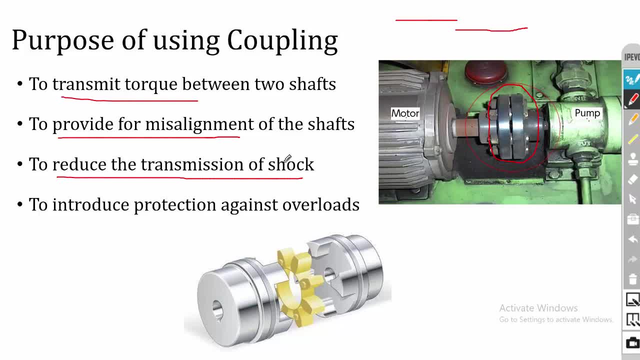 to the generator. so in that case some flexible couplings, like bush pin couplings, are used in between the generator and the engine. So there the couplings are absorbing some amount of vibration. so it's all about absorbing the vibration and damping. ok, so damping means it is the reduction of vibration. so in that, 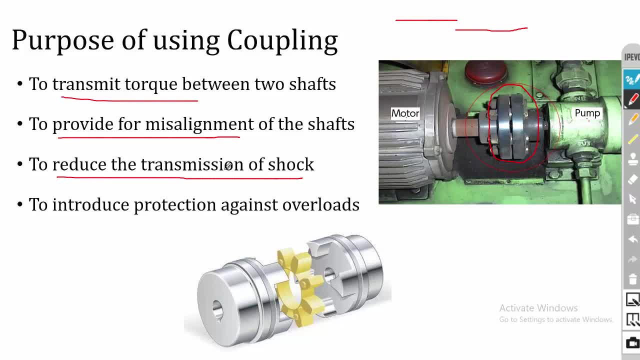 the vibration generated in the engine will not be transmitted to the generator. The last one is to introduce protection. so this is the example for a flexible coupling. so here you can see that some rubber component is there. so this part is connected to the engine And this part is connected to the generator. so the shock generated in the engine will. 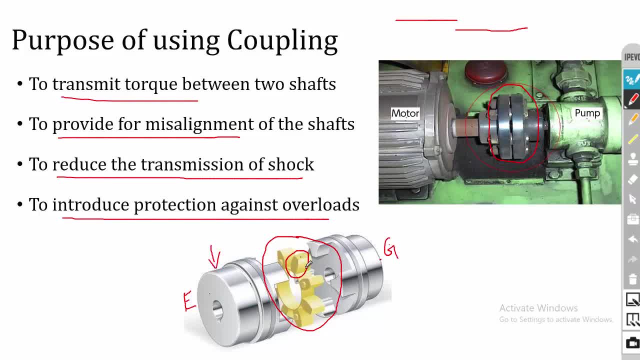 not be transmitted to the generator, because this rubber component will absorb the shocks and only the torque will be transmitted to the generator. Then the last one is to introduce protection arm against overload. so when one component is subjected to overload, so this couplings will absorb some amount of loads and it will 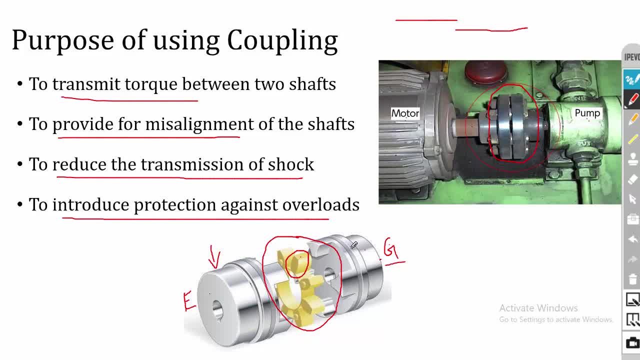 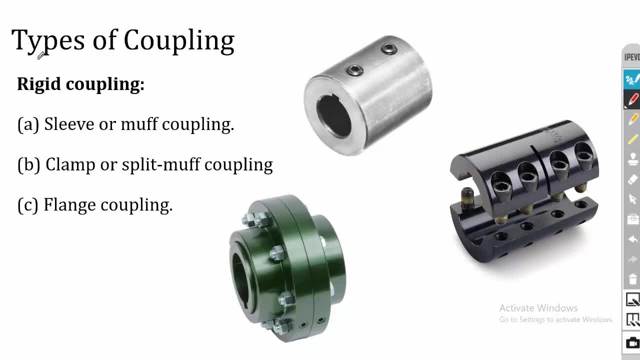 transmit only the desired load. So this is the purpose we are using for coupling. so there are many types of couplings, are there? the couplings are classified based on two types. one is rigid coupling and another one is flexible coupling. there are three types of rigid couplings are there. one is sleeve. 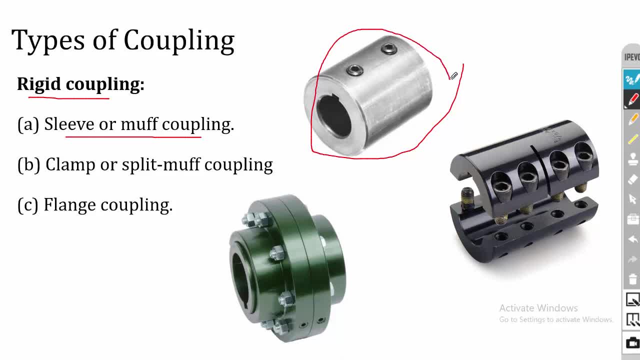 or muff coupling. so this is the sleeve coupling. so this is almost like your plumping coupling. so in your plumping pipes you might have seen the couplings. so the coupling is a hollow circular one And in that coupling two pipes are inserted. so similarly for muff coupling, two shafts. 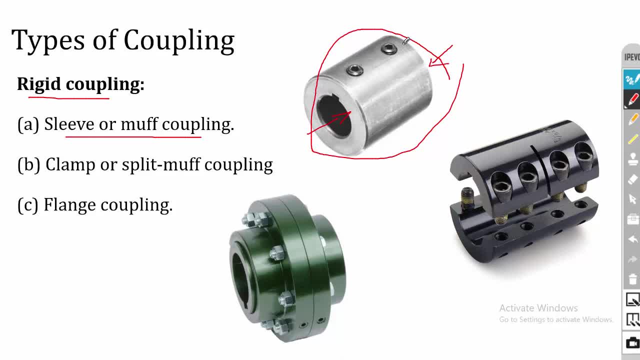 will be inserted and a threaded fastener is used to connect the two shafts, so the power is transmitted from the shaft to the hub and from the hub to the another shaft. So this is a muff coupling. this is a hollow circular shaft, that's all. 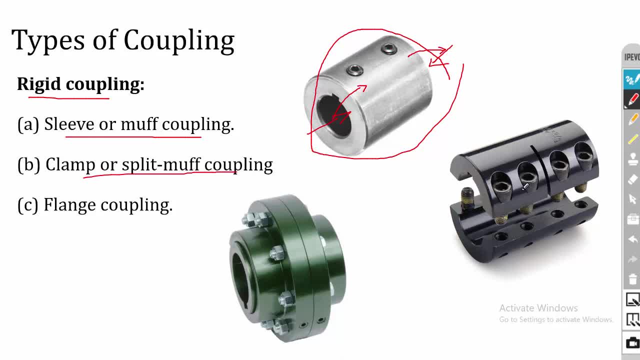 Then the next one is a clamp coupling or a split muff coupling. Ok, So here the muff is split into two halves, so upper half and lower half, so it's almost like a clamp. so that is why it is called as clamp coupling, in that the shafts are inserted. 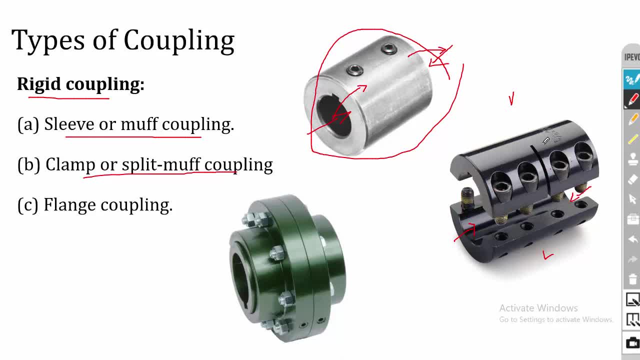 in the coupling and the bolts are used to connect the two parts of the coupling. so this is the second type of coupling, that is, clamp coupling. and third one is flange coupling. the flange coupling is the most important one and in 90% of the applications the flange 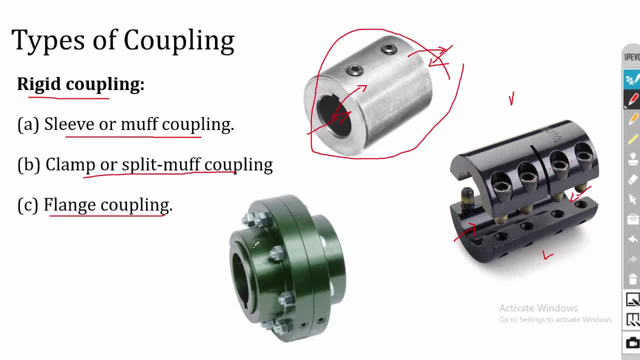 coupling will be used. So you can see two flanges. ok, so this is the flange of left side and this is the flange of right side. so the left side flange is connected with one shaft using a key. you can see that a keyway is there. ok, so the key is inserted between the shaft and the coupling. the key. 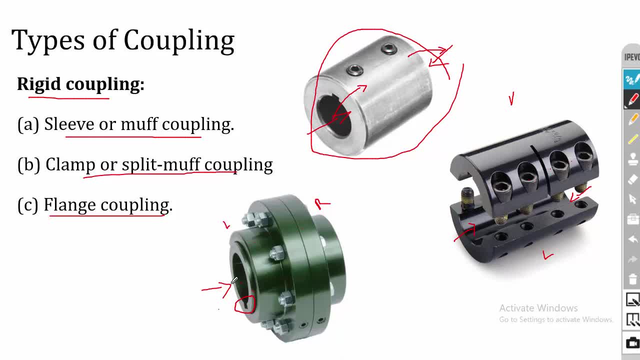 resists the relative motion between shaft and the coupling. so the power is transmitted from the shaft to the key to the coupling and the next flange is connected with the left side flange using the bolts. Ok, So the bolts are used to connect the two flanges and this flange is connected with. 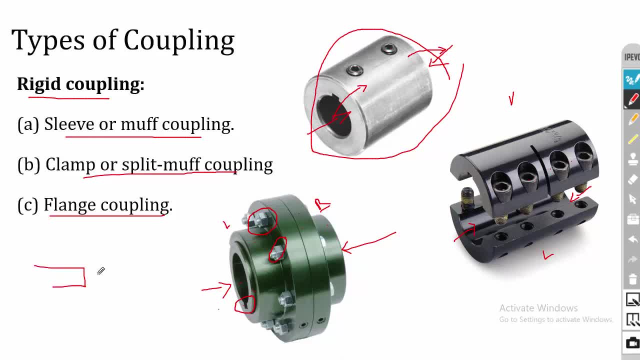 the another shaft. you can see that. so this is a shaft and this is another shaft. so here two flanges are used. this is flange number one and this is flange number two. So these two flanges are connected with this shaft using a key. 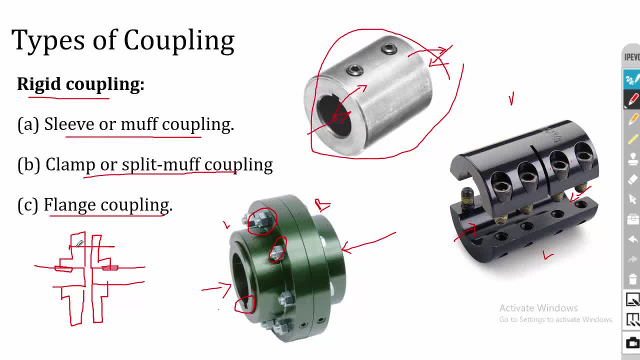 and these two flanges are connected together by using some bolts, And this is a flange coupling. So flange coupling is used to transmit high amount of power and at high amount of speed. the next one is a flexible coupling. so in the case of flexible coupling, the flexible. 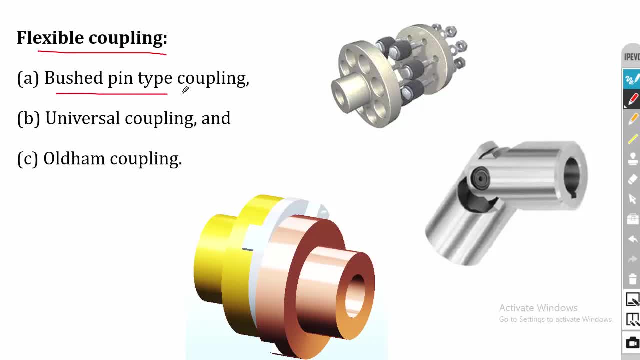 coupling will provide some flexible movement. the first one here is a bushed pin type coupling, almost a rigid flange coupling, but only thing is a washer or a bush is used in the bolt. So in the rigid coupling the bolt is directly clamped. here some rubber material like bushes. 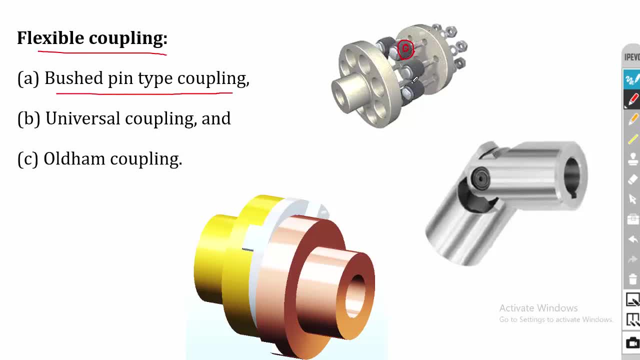 are used in between the flange and the bolt to absorb some amount of the vibration, So this will act like a flexible one. and the second one is universal coupling. So this universal coupling is used in the automobile propeller shaft. The propeller shaft in automobile is used to connect the power from the gear box to 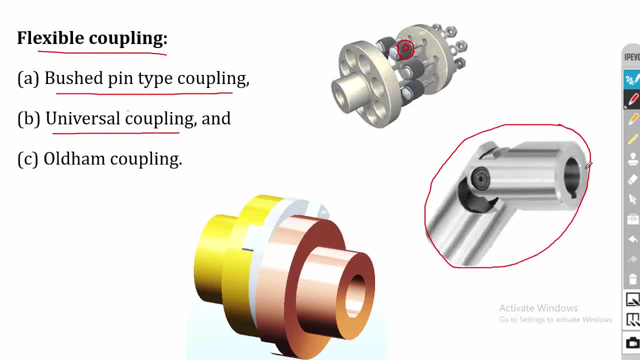 the differential. So there the universal coupling is used, and the universal coupling will transmit power between inclined shaft. The flange coupling will not transmit power between inclined shaft, but this universal coupling will transmit power between inclined shaft. And the last one is old ham coupling. 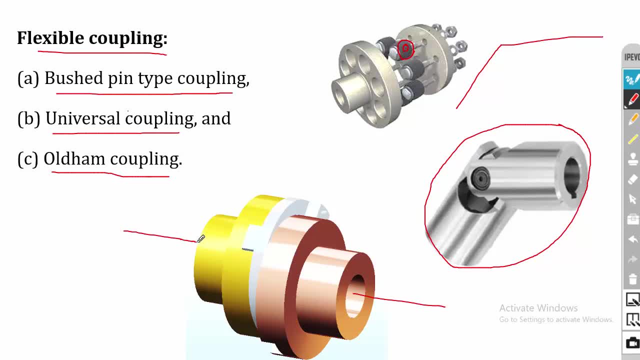 So this old ham coupling is used to transmit, Transmit power between non collinear shaft. So if one shaft is like this and another shaft is like here, then you can use the old ham coupling, but the shaft should be parallel and no need to be collinear. 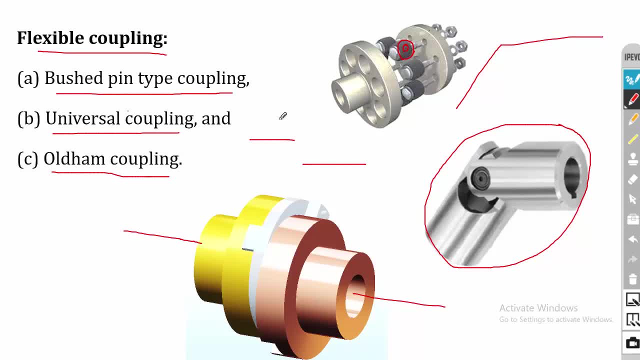 So this old ham coupling can be used in case of in case to avoid the effect of misalignment. So these are all the three types of flexible coupling. So in our subject, first we are going to start with the design of flange coupling, then we 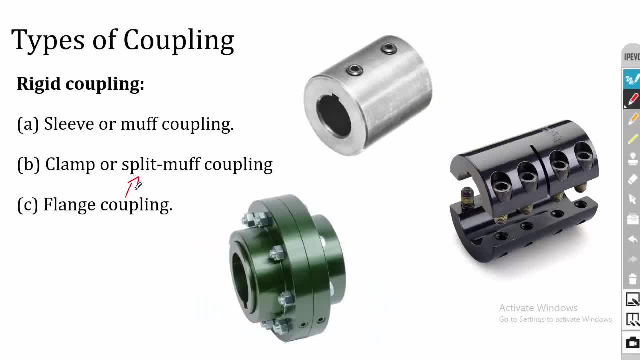 are going to move, for In the return we are going to move. So first design of flange coupling, then the design of split muff, and from the split muff we are going to design the muff coupling. Because once if you design the flange coupling, then the split muff and muff will be very easy. 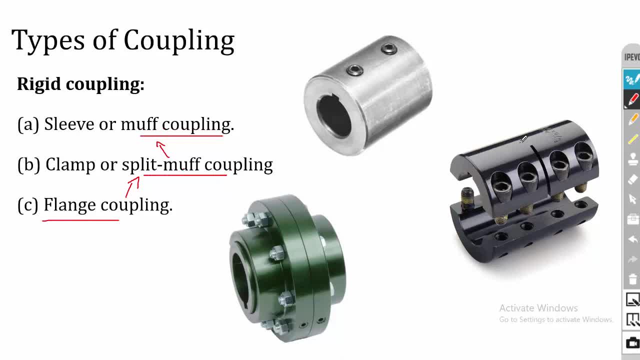 You can see the image in the flange coupling there are many components are there, But in clamp coupling only the clamp and bolt is there. In the case of muff, only a hollow circular shaft is there. So first we will focus on the design of rigid flange coupling and flexible flange coupling. 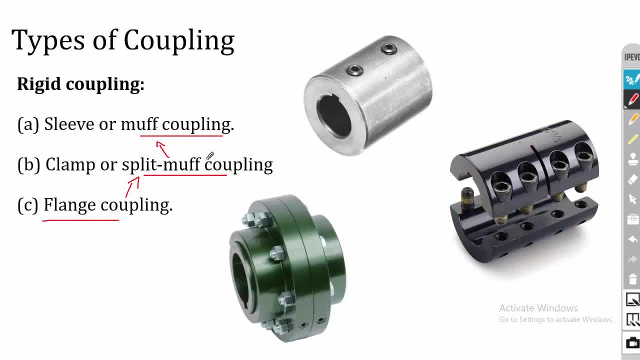 Then we will move into the design of split muff and the muff coupling.